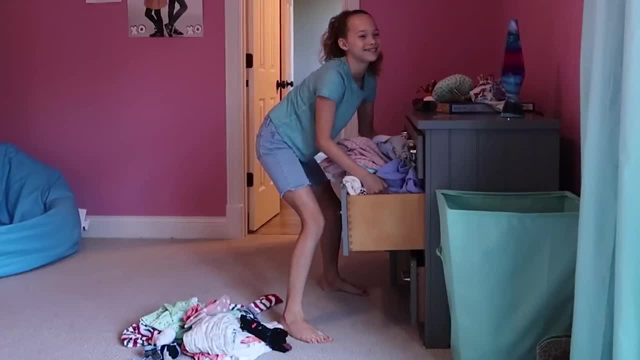 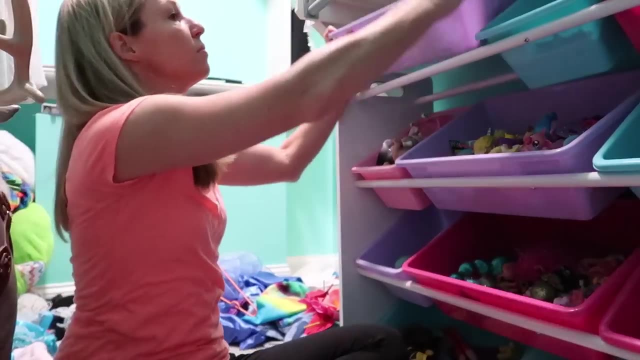 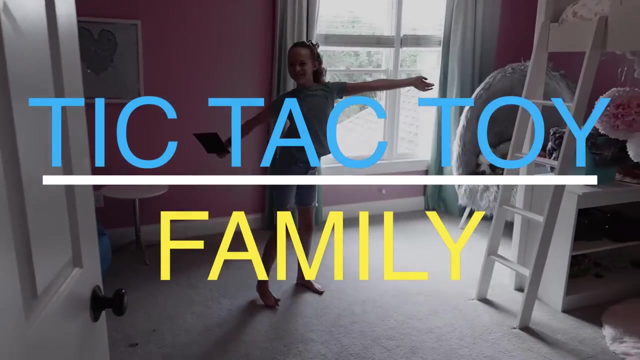 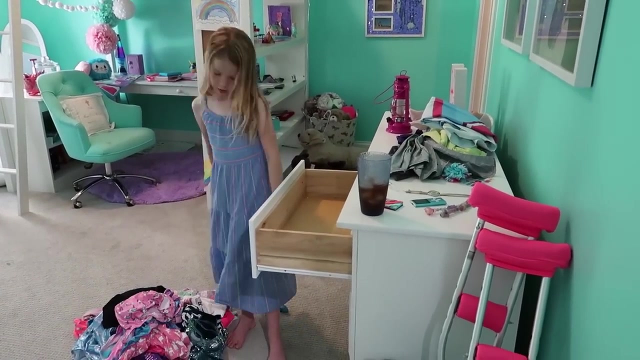 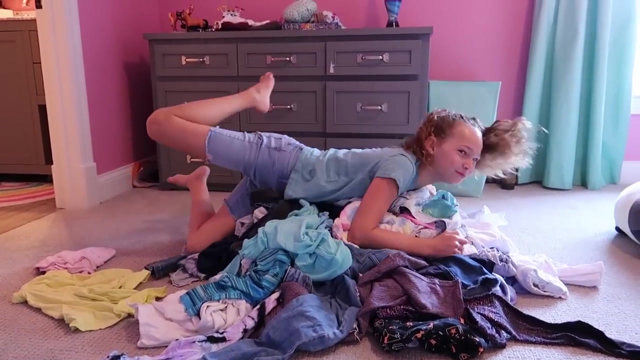 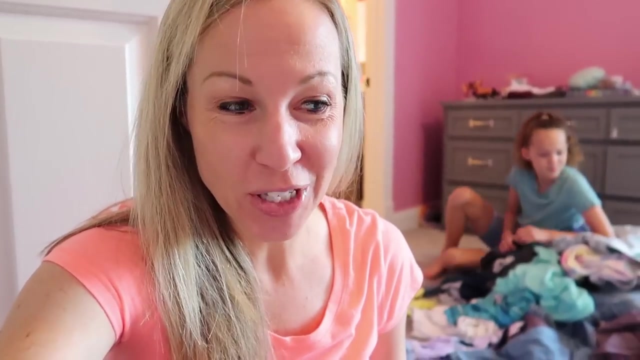 And we'd love to see you there. so make sure you subscribe. Keep going, all the drawers empty. All of this was in my dresser, My goodness, Addy. Today we are tackling something that I have wanted to tackle for a really long time, and that is going through the girls rooms from top to bottom, one end to the other end. 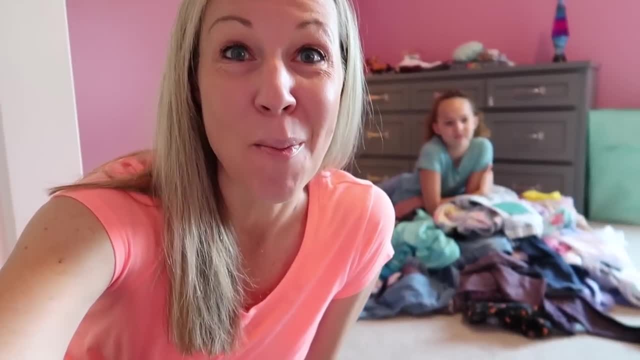 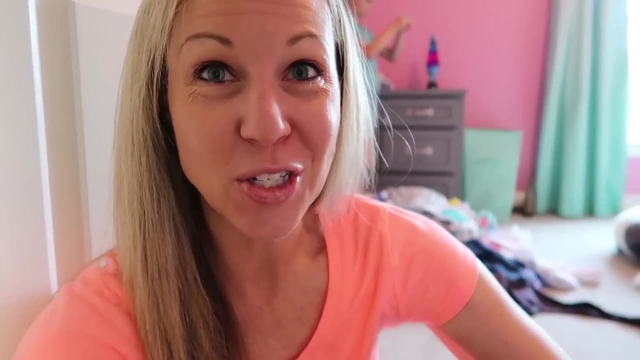 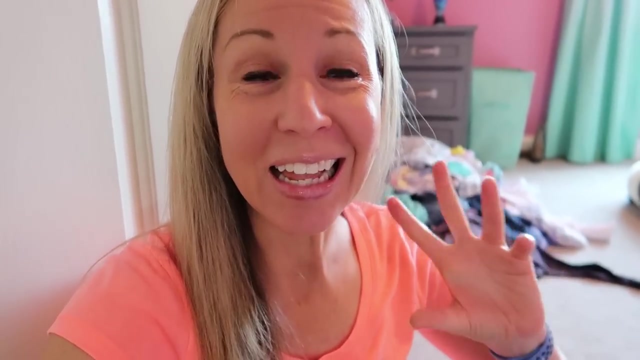 to the dressers, the closets, the bathrooms and doing a major, major clean out and organization day. every time I walked the girls room for the last six months I like still panic attack inside of me because they are so messy and just cluttered and I just I can't even take. 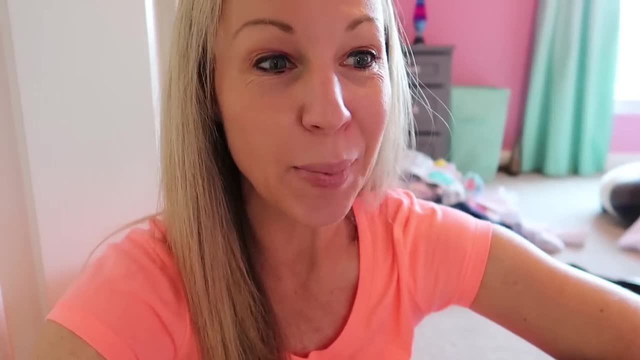 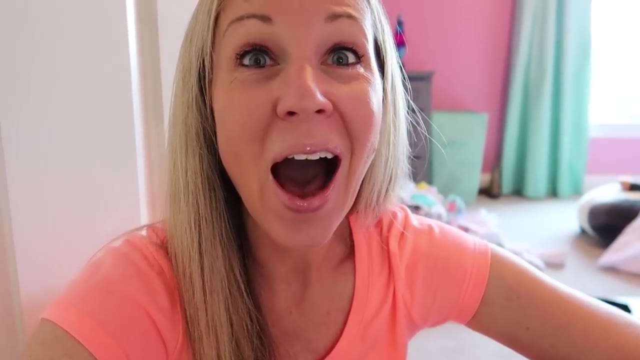 it. so I kept telling myself this summer we're gonna take a full day and we're gonna do it. and before you knew it, this summer is like almost over. so I found a day this week to do it and I have to tell you I have been trying to psych. 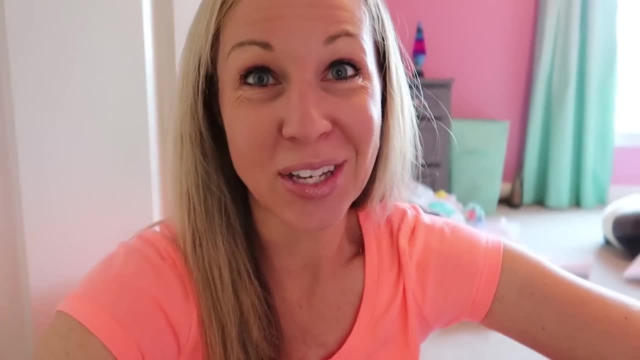 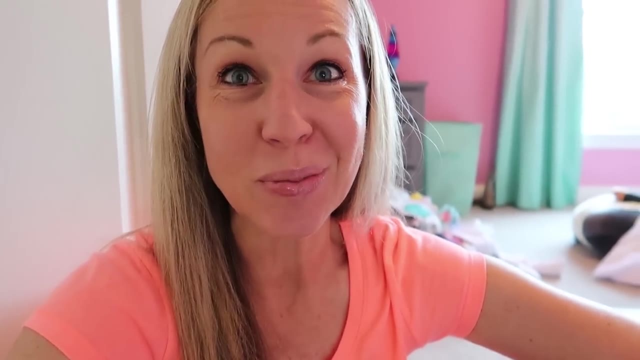 myself up for this day mentally all week long, because I know it's gonna be a long day and it's gonna be an exhausting day and it might be a little bit painful, but we're gonna get these rooms cleaned, get it all emptied out, Maya, yeah, every. 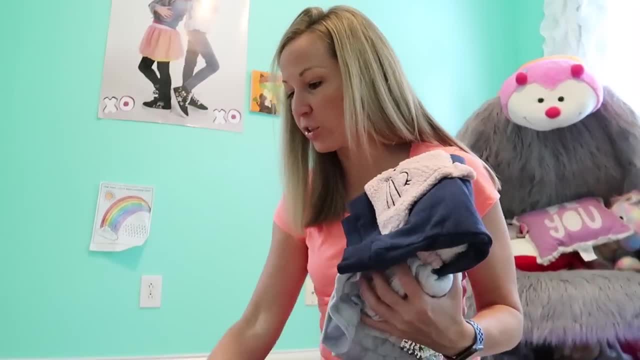 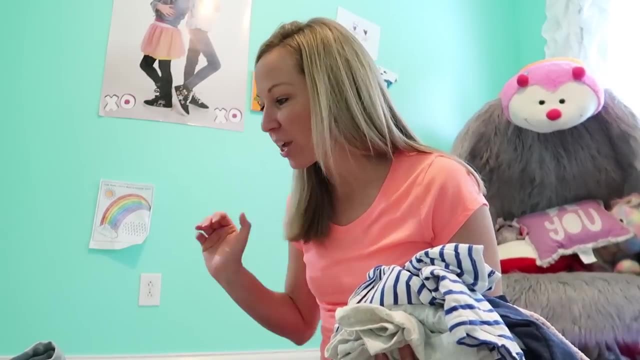 article of clothing. the first thing I wanted to do was have the girls go through all their clothes, because we have quite a collection of things of use for different videos, things of use for various projects and I'm sure a lot of this they've outgrown doesn't fit them. 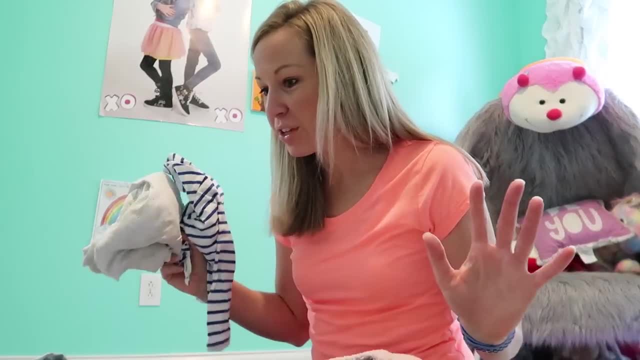 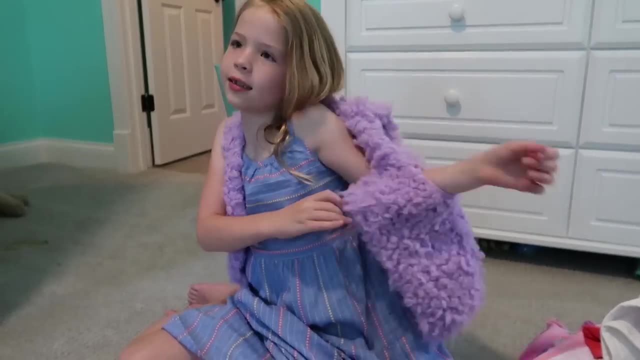 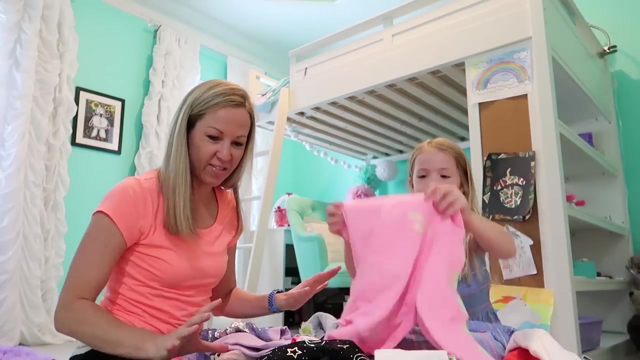 maybe they're stained or dirty, we're done with them. so we're gonna go through these clothes and clear out and donate- yeah, that you haven't worn in a long long time, okay. so, Maya, we're gonna go through these and we're gonna purge more than half of this. we're gonna donate. you got it. so, for example, you wore this on: 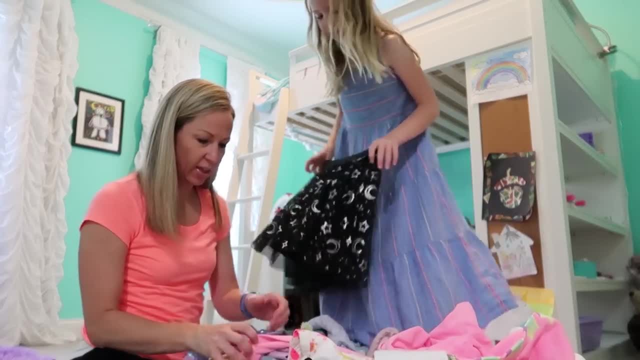 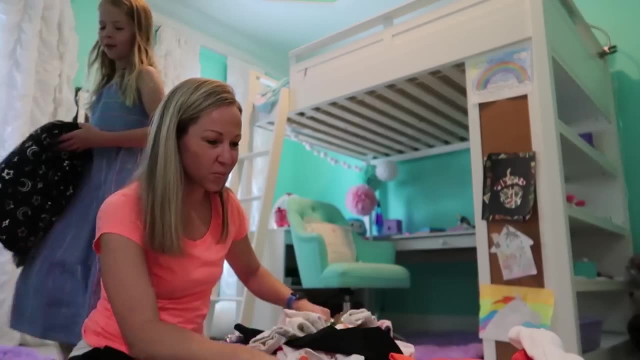 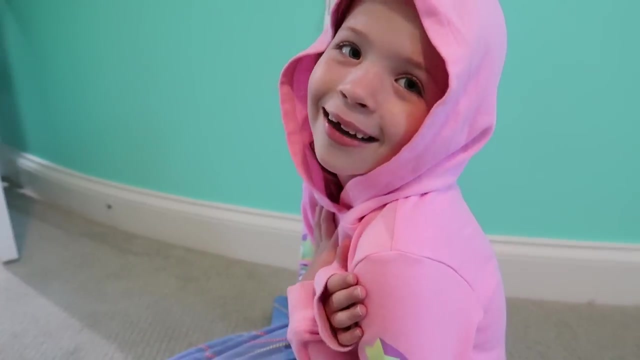 Halloween, but I don't think you've worn it since. I think we can donate that. it has a hole in it. we can get rid of that. oh, Maya, so that's the key. okay, if that's a keep that find that. we have to find a lot. 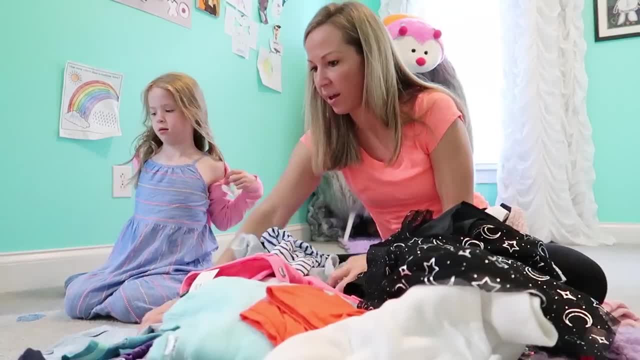 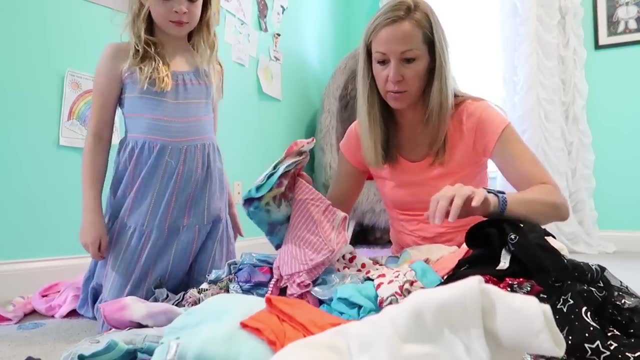 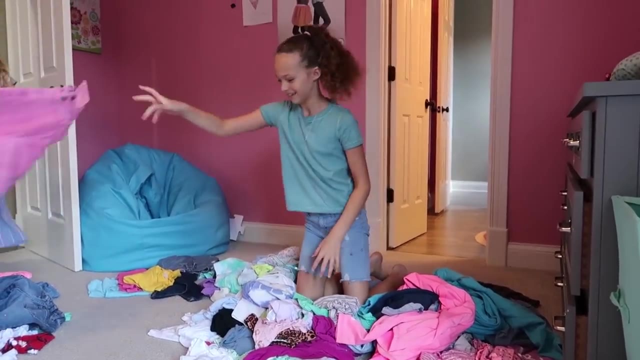 more that we're willing to get rid of this. we're gonna donate that. if these are old, we're gonna donate these. I know they've served you well. I forgot about this. this is so old. you can donate it. you can donate it. all. right, Maya, I think you're putting more. 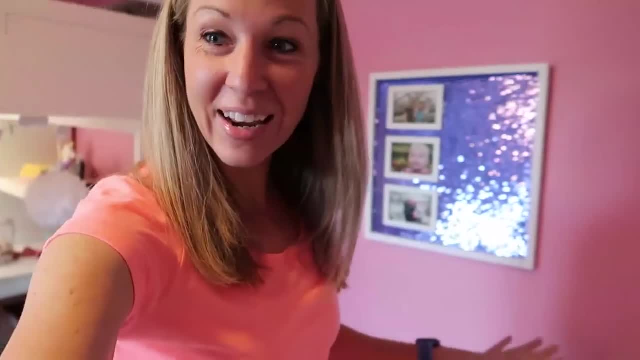 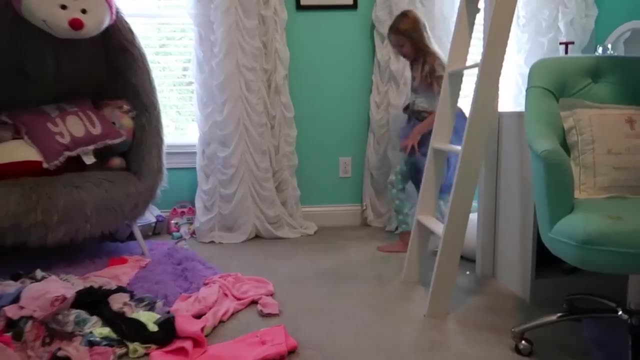 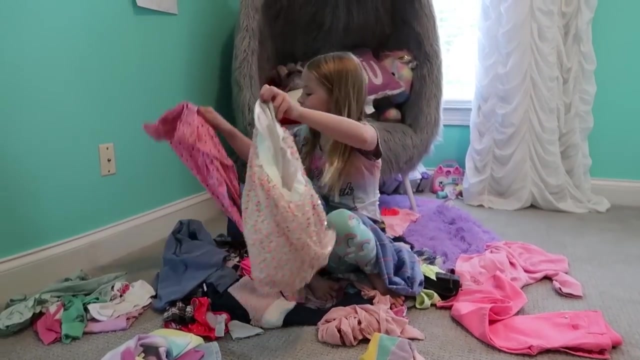 clothes on then we're getting rid of. let's go back to your room and you keep working. girl Maya and I are heading back to her room to continue going through her pile of clothes. oh you taking some of Addie's pants. yeah, I think Maya's pile of clothes is growing. 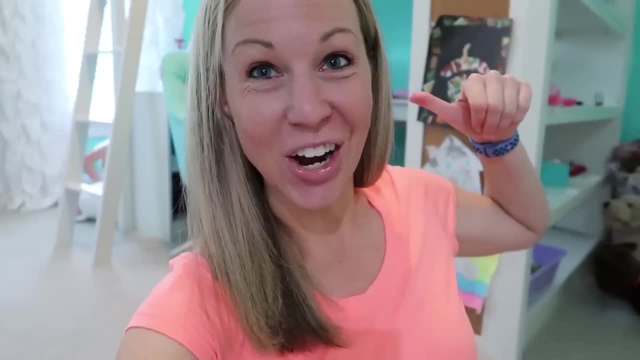 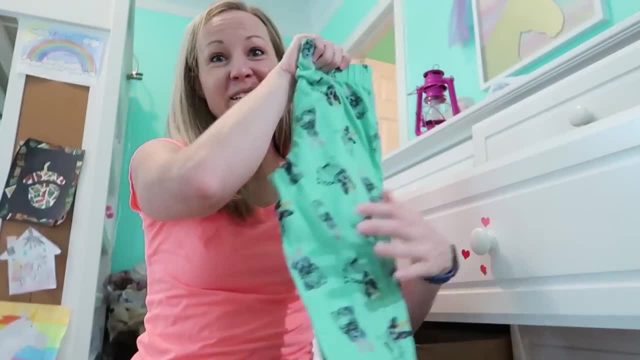 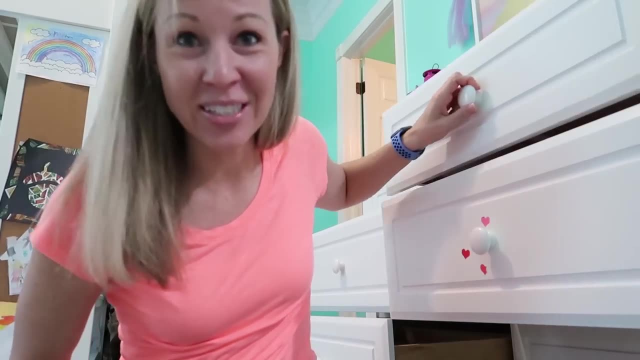 reasons I decided to vlog this experience today is because I needed the accountability. I knew, if I was gonna do this on my own and I wasn't making a video, that there was a good chance. I would just tire out and give up and I leave a giant mess in the room and it's there for a week. but now that I'm 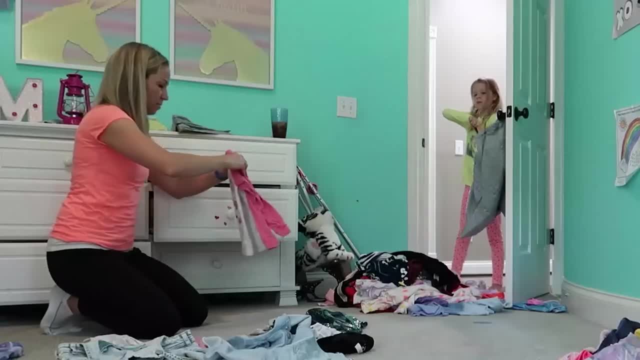 filming it. I know that I have to get this done. I have to get these rooms finished today so we can show you an end product, and I know that I have to get this done. I have to get these rooms finished today so we can show you an end product. so we can show you an end product. 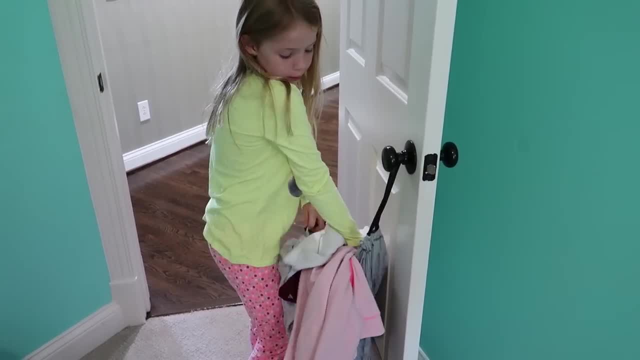 and it's just gonna give me that extra motivation to get through this as quick. and it's just gonna give me that extra motivation to get through this as quick as we can. I told Maya, if you say no to me for this one which we used in a 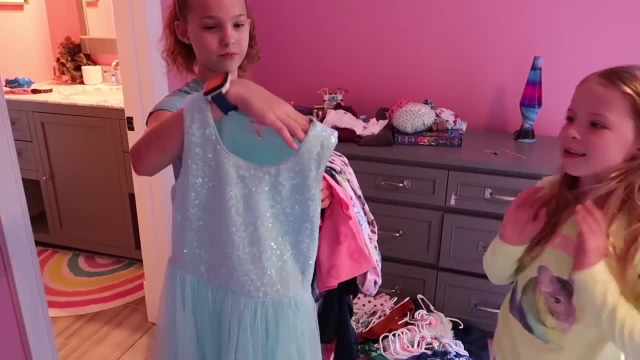 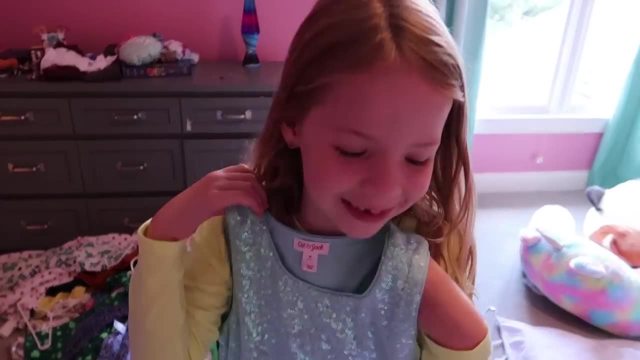 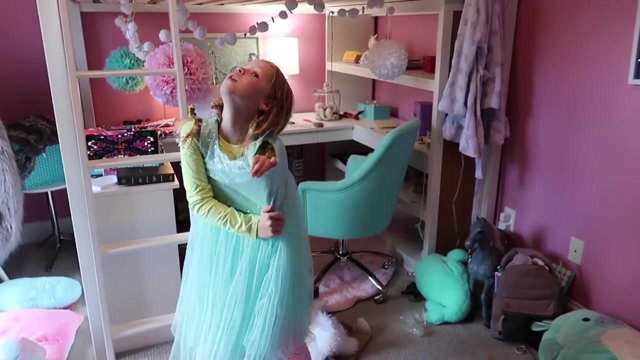 celebrity like toy cafe video. oh, we did use that. I remember that for you. so can Maya have it? you want it, Maya, dressy? sure I like this dress for church. that is a pretty dress for church, Maya. how many layers of clothes do you have on now? 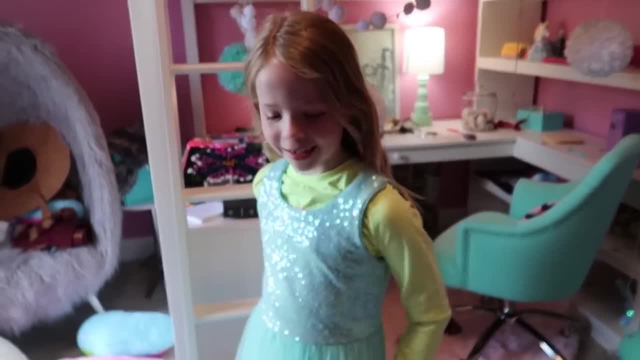 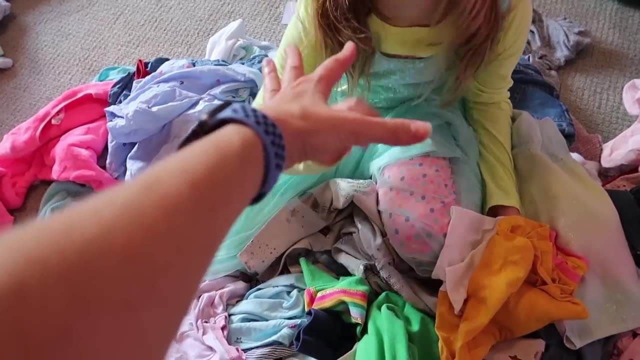 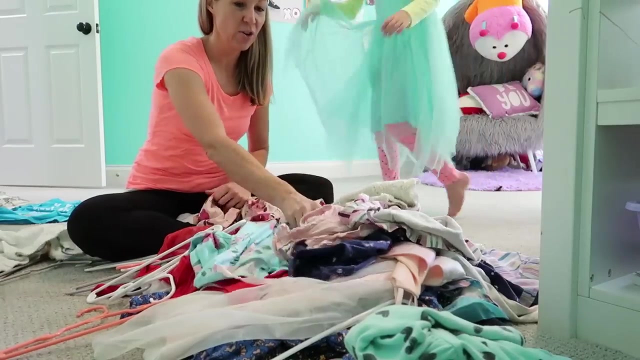 Pants, Shirts, Dress. Okay, Maya, I lost you. back with me, back with me. take my hand back to your room. girl, no more clothes for you. you've got plenty, alright, and you? now you need to help me get all these dresses back on hangers. the good. 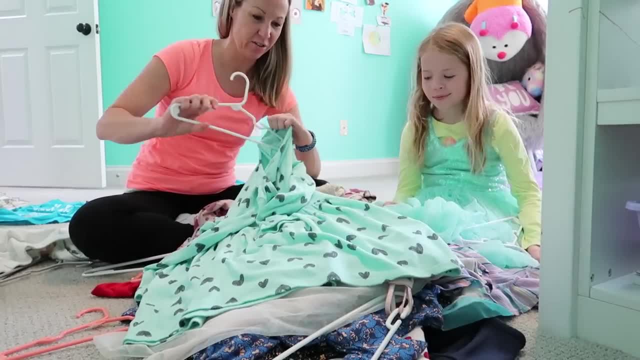 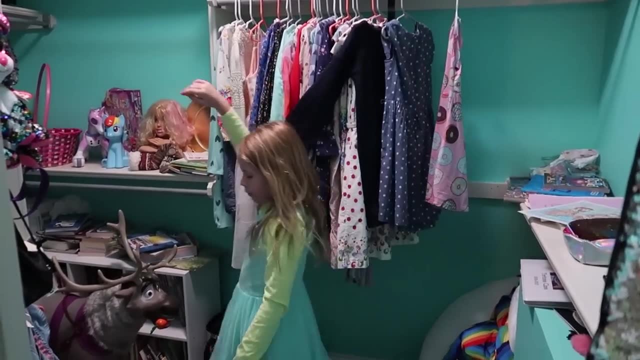 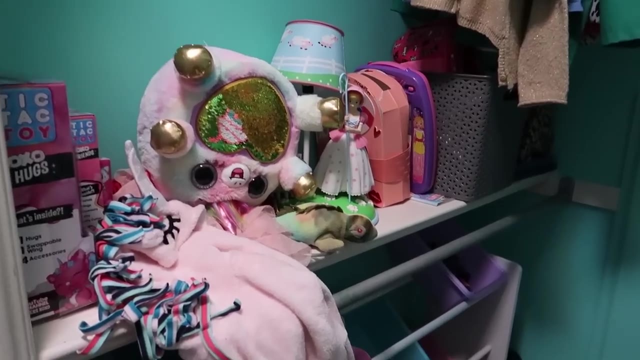 thing about having a big sister is: you've got a lot of hand-me-downs, don't you? girl, girl, now that we've got most of my clothes done, we have. this is her closet guys, and oh, this is what we got to tackle soon. not to mention, we haven't 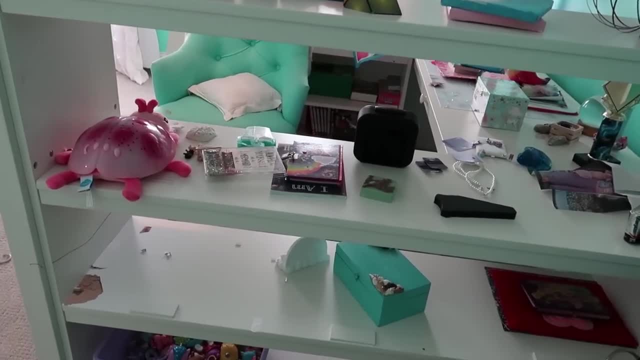 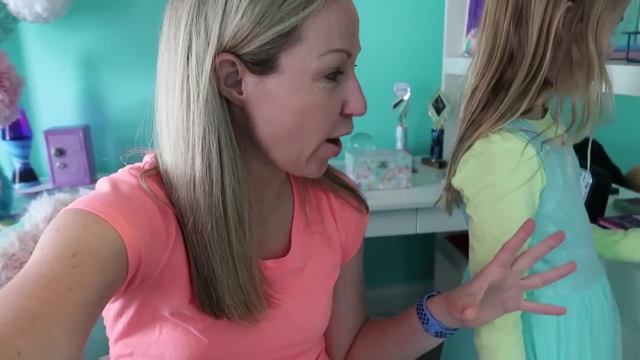 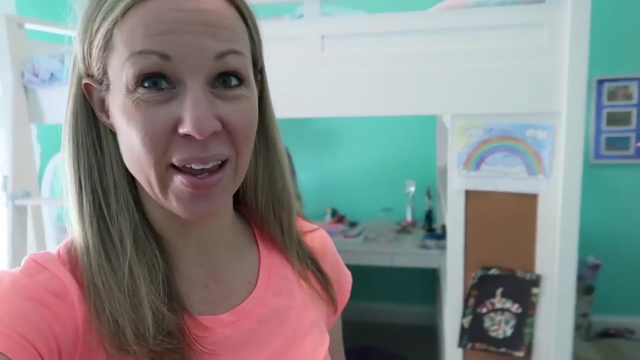 even done the rest of her room yet. I can't bring myself to tackle the closet yet. that's just a little bit overwhelming. so we're gonna tackle my loft bed, this desk area, right now, because she's got a lot of stuff on it. now. one question we get asked all the time, we get lots of emails about, is: 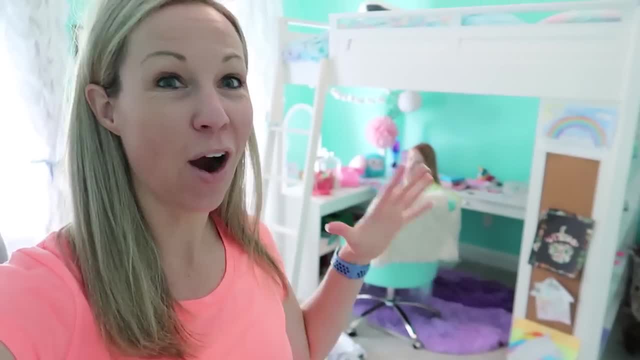 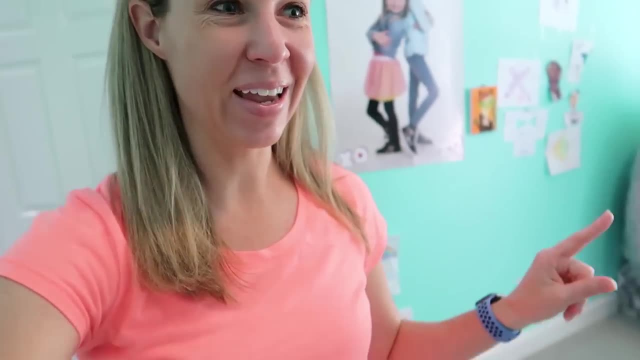 where do we get the girls? loft beds. a lot of people love them, they are a lot of fun. and then I tell you that they're from Pottery Barn teen. we love them absolutely, but the one thing I will say is that it has a lot of open storage for. 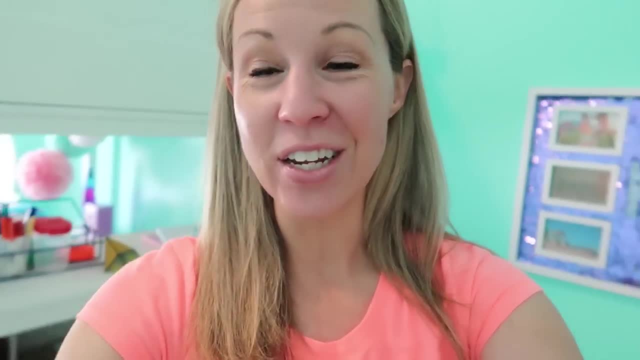 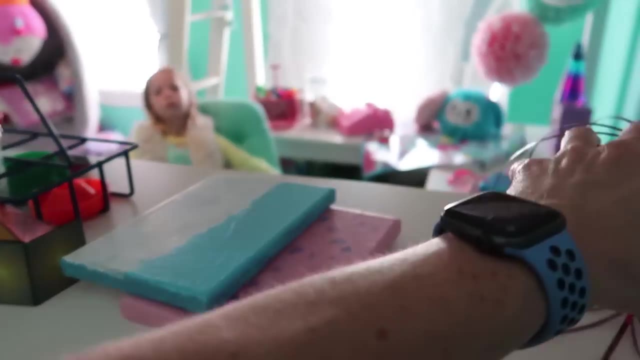 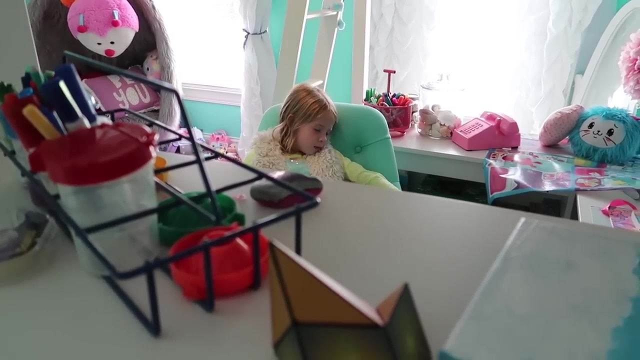 kids like all these shelves and open storage is fun, but it gets pretty messy looking with kids just piling stuff on there. so that's the only thing I would caution you about is the open storage. open storage is difficult. you gotta get up and come help me, girl. up, up, up, up we. 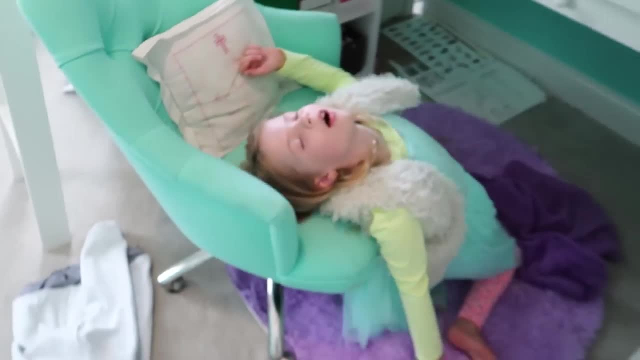 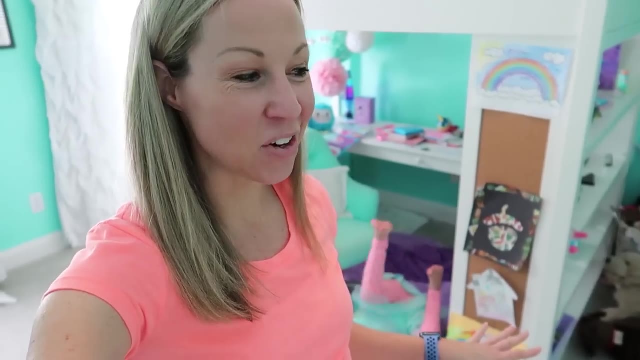 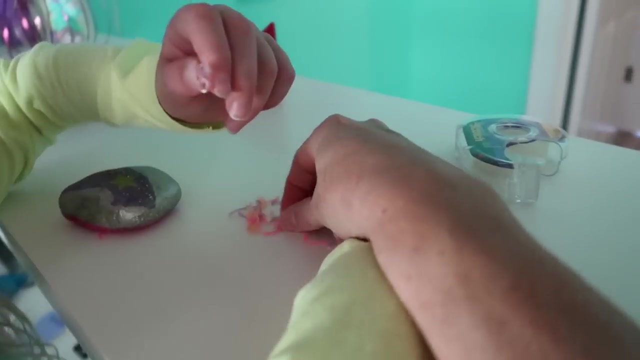 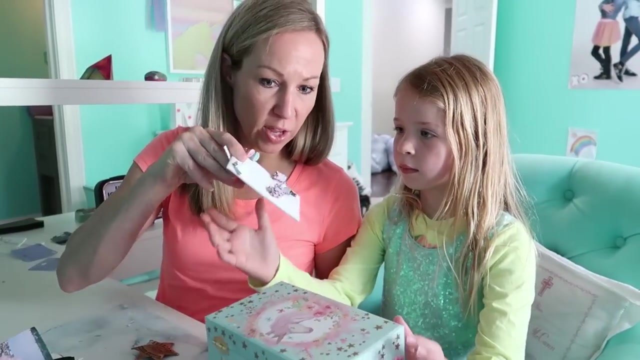 go, she can tell my it's not a big fan of cleaning out and organizing her room. bracelet that got melted. okay, you can definitely throw all that away then. okay, but you have a jewelry box. I need to gather up all your like little pieces of jewelry that you have. 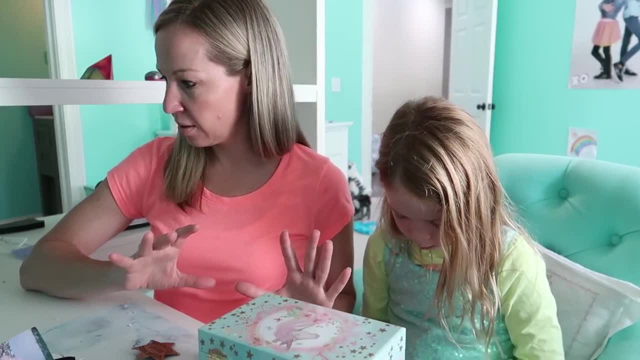 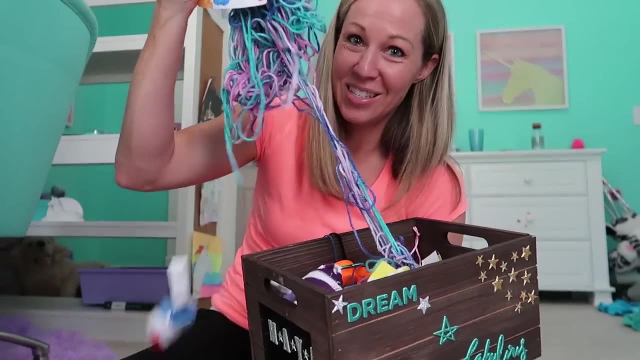 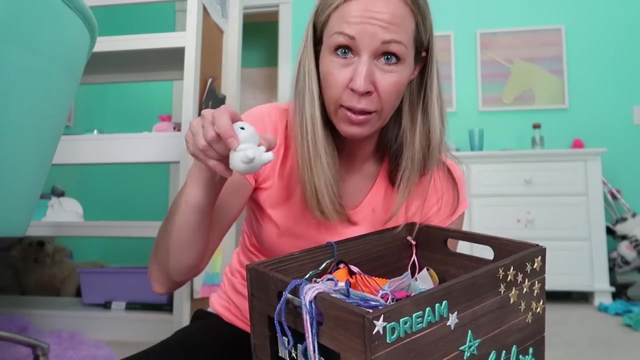 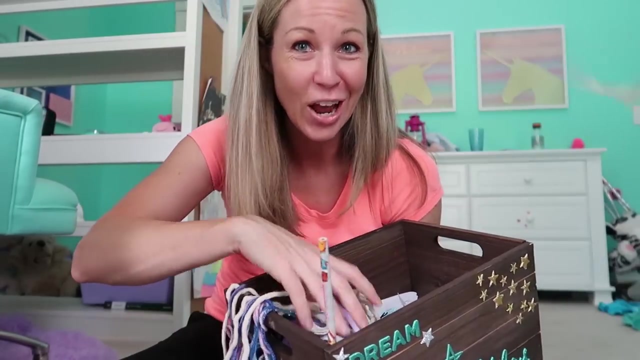 sitting around and let's store all those inside there, okay, okay, this is the kind of stuff that stirs to drive me crazy. we just have bins filled with brain quests, a yellow sock, a little now, some flashcards, all little, just like sorts of stuff and new things. drive me crazy. 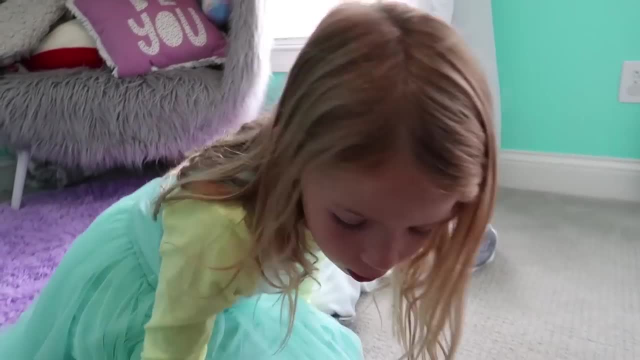 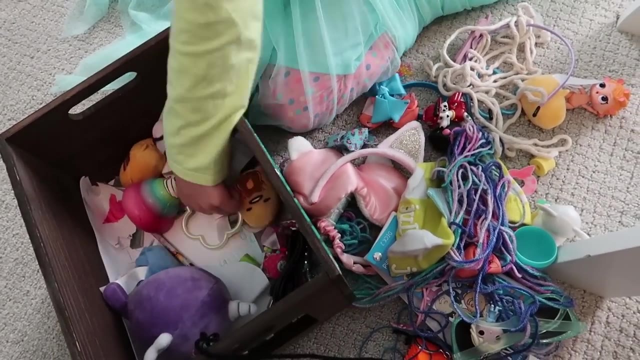 What is all this stuff? Just a Воcher. What is all this, Maya? I don't know, You don't know. Can we sort it out? Sure, Maya is a little bit of a pack rat. Are you a pack rat, Maya? 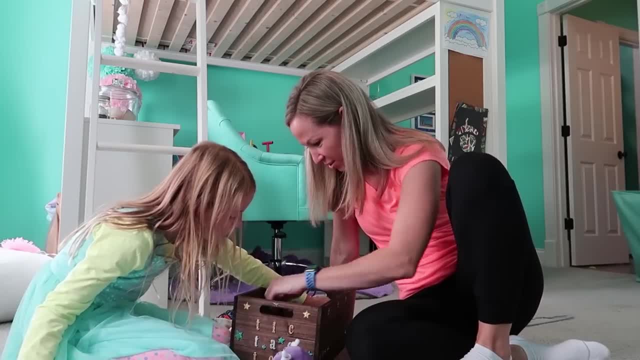 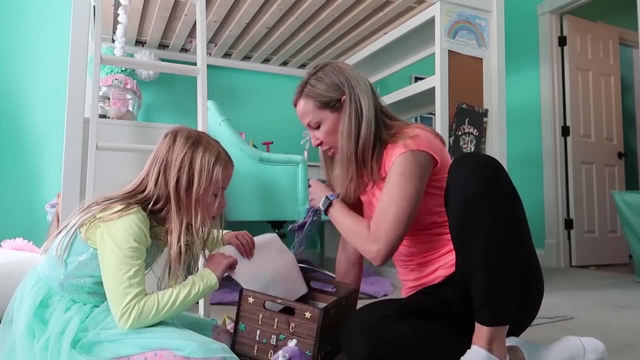 I don't know what that means. You don't know what that means. It means you like to keep everything, I guess so. You guess so We could say she's sentimental. We'll say that, instead of a pack rat, You're a very sentimental person. 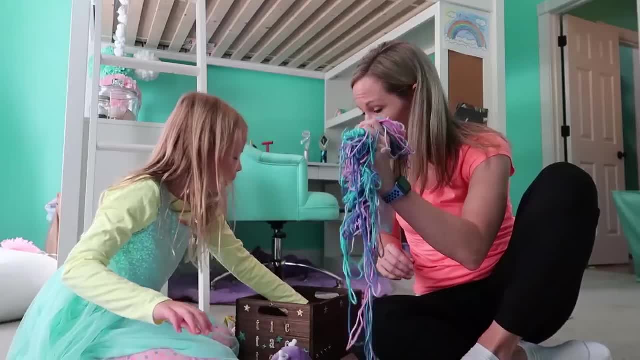 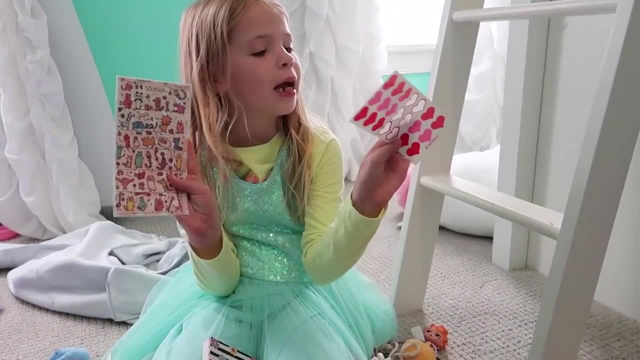 Every little thing has value to it, And we have a hard time parting with things. I've been looking for that, You've been looking for that. Well, you found it. Ah, my stickers. Here they are. I finally found them. 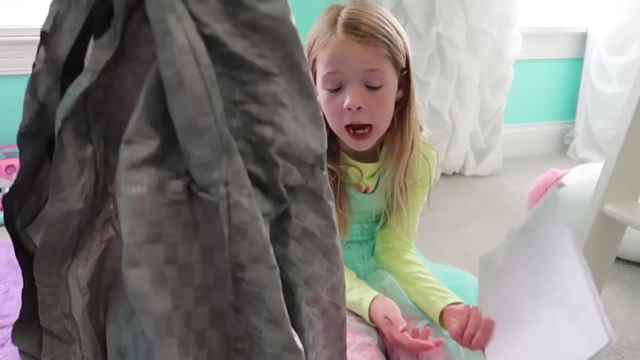 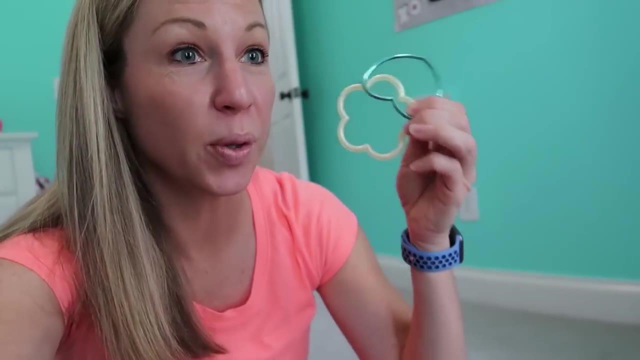 Do you know what this is? Uh, no, What is this? I don't know. Yes, you do. Well, I want you to really think, Maya. For example, do we really need these little bracelets? Yep, Do we really need this little bag? 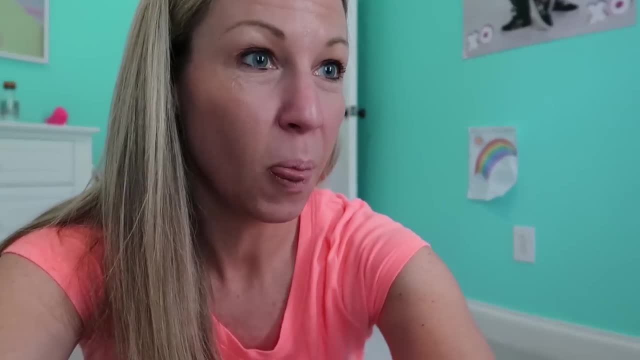 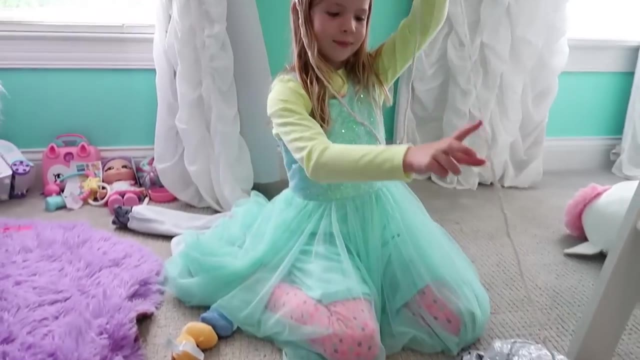 All these little things. Really think about what can we get rid of? Nothing, Nothing, Nothing. I don't think so, girl, You gotta get rid of some of this stuff. This is where Maya and I are very different. As I said, Maya's very sentimental. 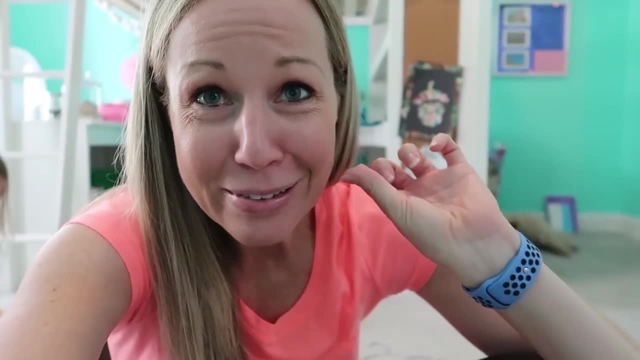 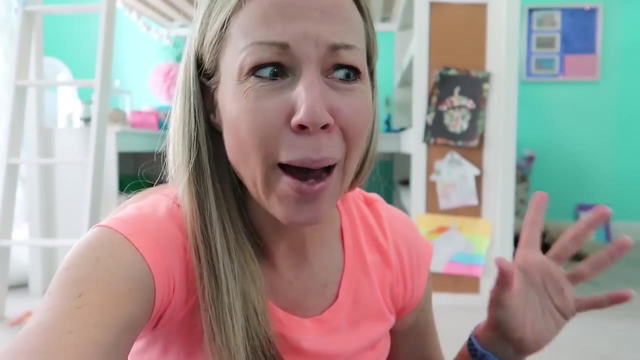 and she likes to keep everything, and every little token of little tiny toy has some important meaning to her, And meanwhile I'm the complete opposite. I am a purger. I'm just not very sentimental about objects and I'd much rather get rid of things. 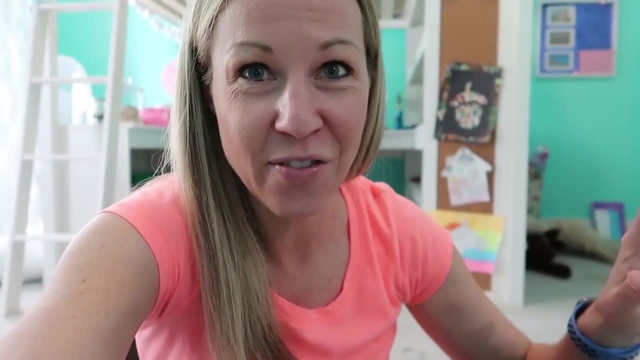 almost to a fault, to the point where I will just purge and get rid of stuff and then I'll end up needing it again, and then I'll have to go buy it again because I needed it when I shouldn't have purged in the first place. 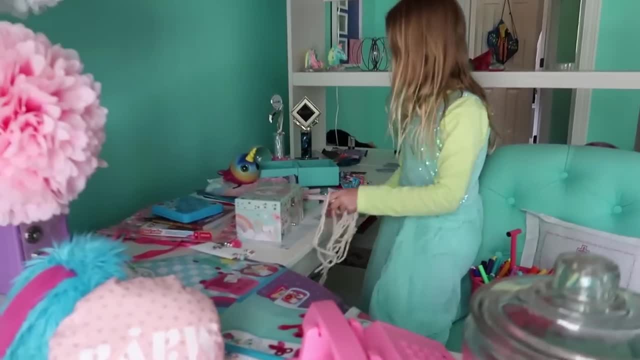 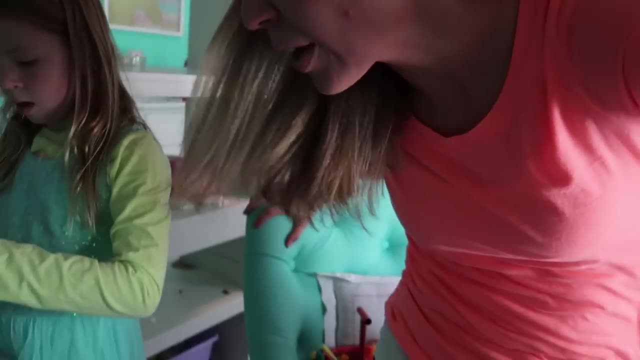 So I'm trying to be aware that we're different, so I don't want to throw away things that are important to her, but at the same time, we need to clean up this room. Wait, wait, wait. Are you keeping yarns like old pieces of yarn? 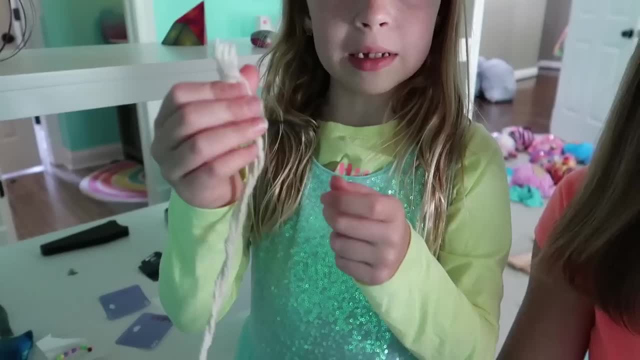 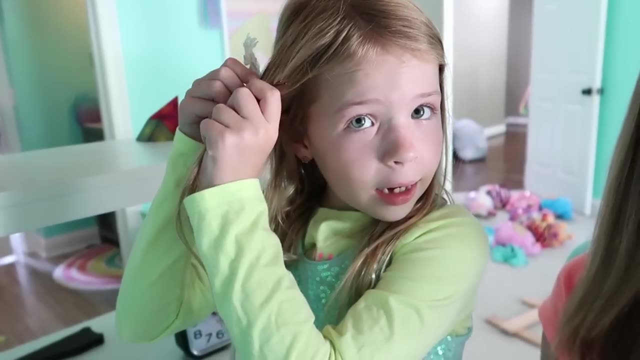 Yeah, What is this? It's Rapunzel hair. see, Yeah, I tied Rapunzel's hair color string to this and that's Rapunzel's hair. Okay, It's jewelry. Okay, we'll keep it. 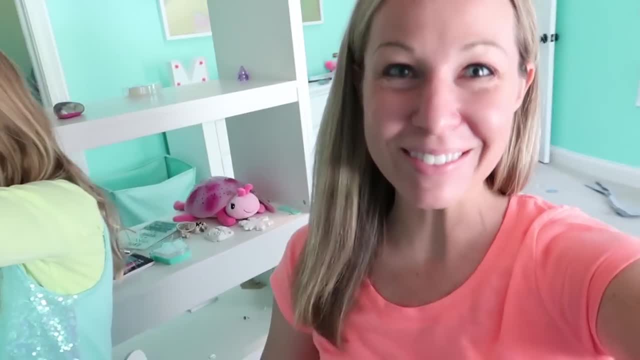 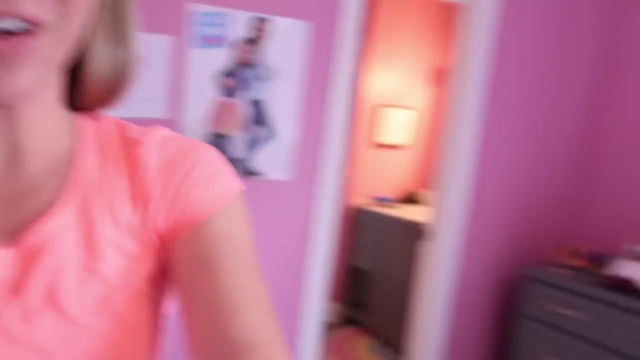 Trash right to jewelry. All right, we'll keep it. I guess we're recycling and reusing. I'm gonna step out of Maya's room and go check on Addy real quickly, Addy, how's it coming, girl? I see a bug. 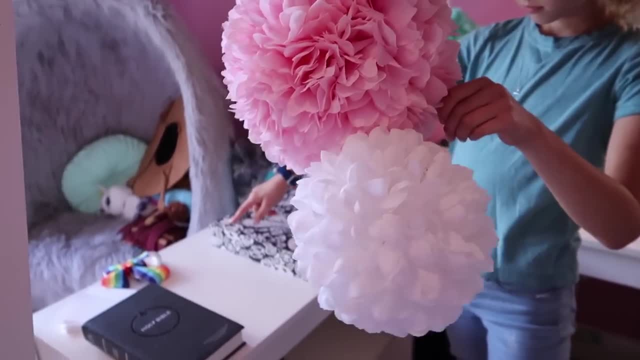 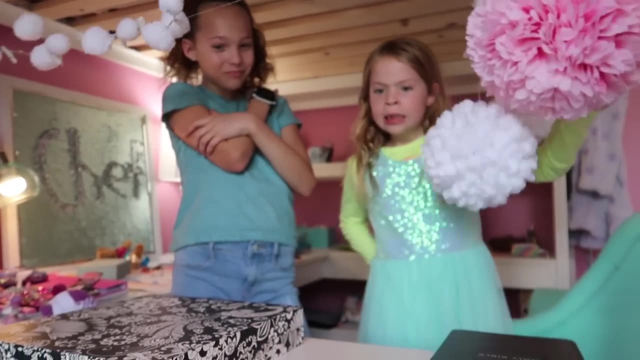 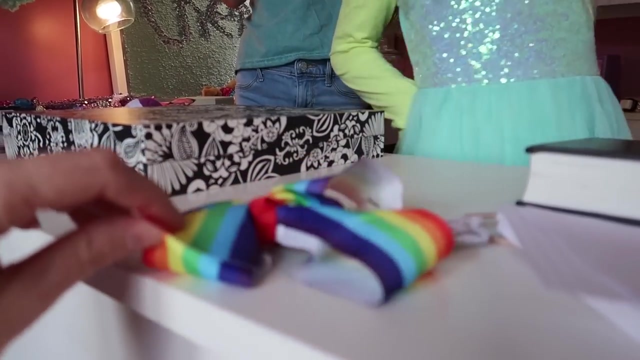 You see a bug? It's right there. Ooh, there is a bug, Bug, bug, bug, buggy, buggy. What is it? It's a mosquito-looking bug in my bow. Okay, let's see here, Let's see. 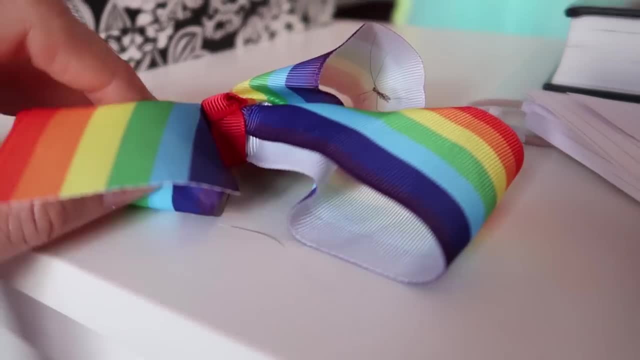 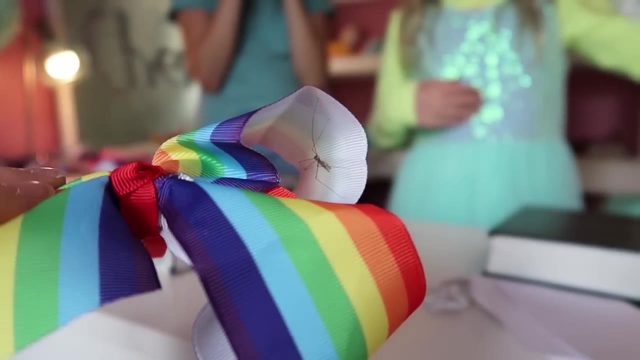 Oh, yep, there's something in there. Mm Yeah, is it even alive? I don't know. but whatever, See, this is our problem. This has probably sat in here. sat here so long that we have a dead bug in your hair bow. 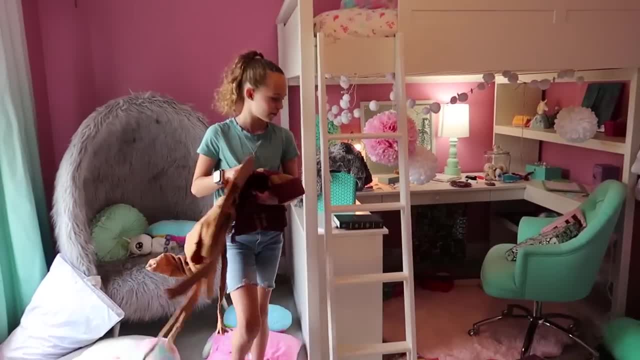 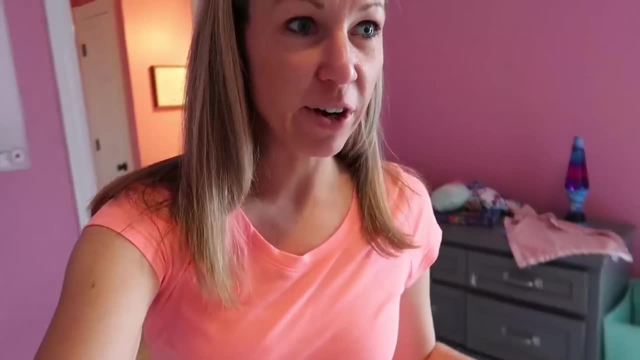 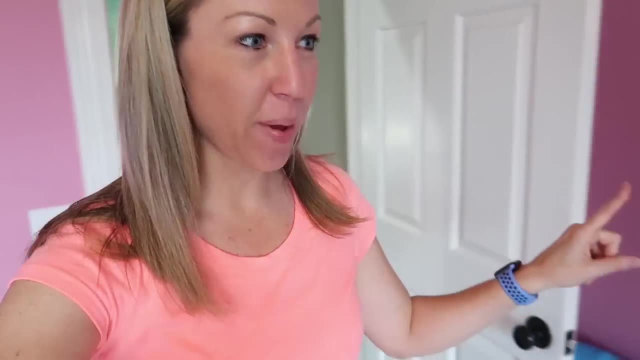 Bug's going bye-bye. Addy, do you have a garbage bag in here? You need a garbage bag too. Yep, Okay, you got one. Yep, Okay, I'm gonna get you a garbage bag, and I want garbage bags filled. 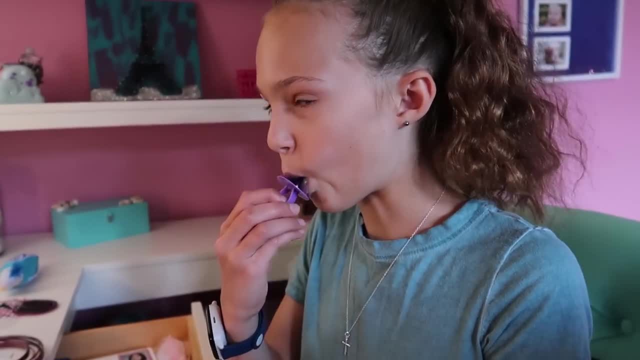 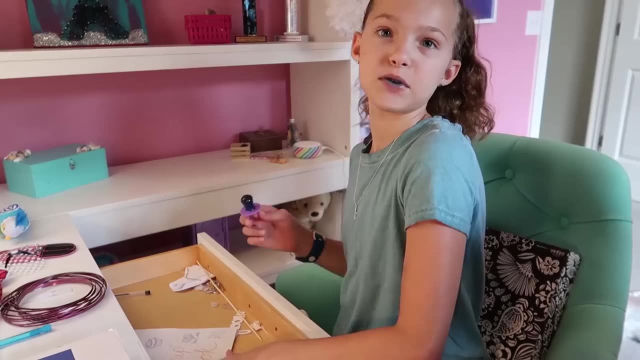 How's your room coming? Good, I see you found a ring pop. Mm-hmm, Yummy, You have a blue mouth now you know that. Yeah, I think in this drawer I'm gonna be like put like craft supplies in my like journal. 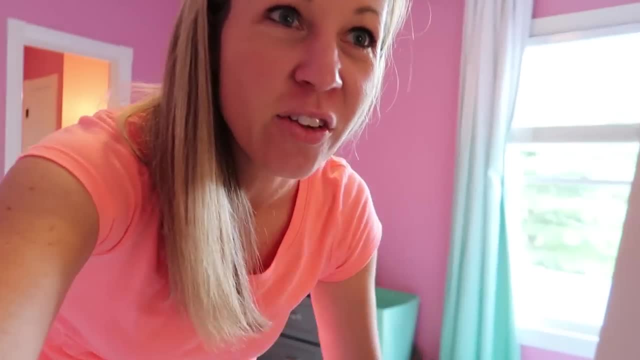 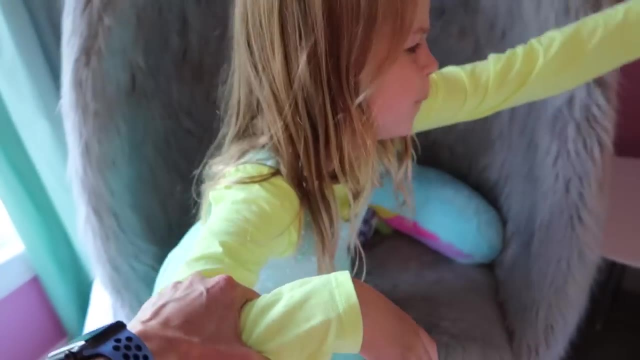 Put like shelf shelves and stuff Your shelves over here are looking really good too. Addy, You've got those really cleared off. What are you doing in here? Back to your room. Back to your room. We have a wandering Maya. 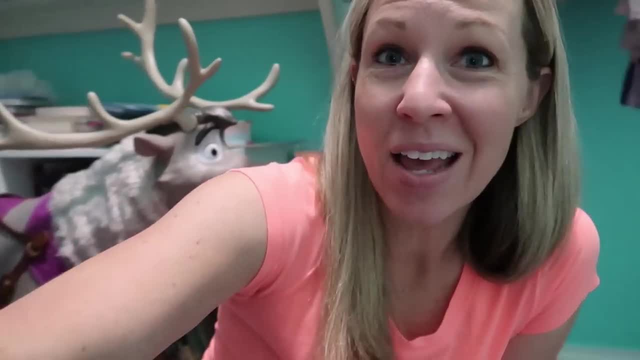 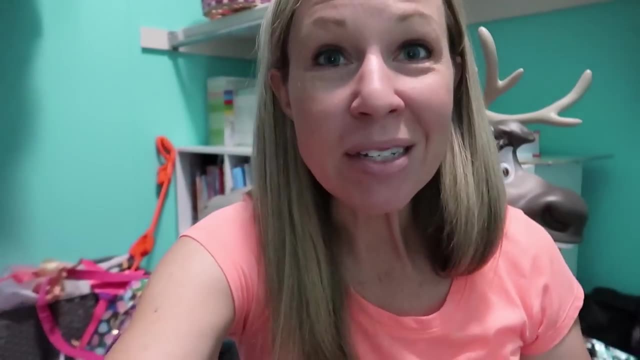 I've moved on to attempt to tackle Maya's closet and, honestly, this is the point where I'm feeling like what in the world did I get myself into? We are three hours into the cleaning process and there's just so much more to do, right? 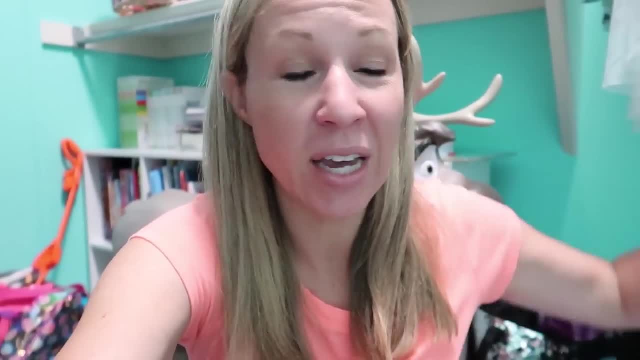 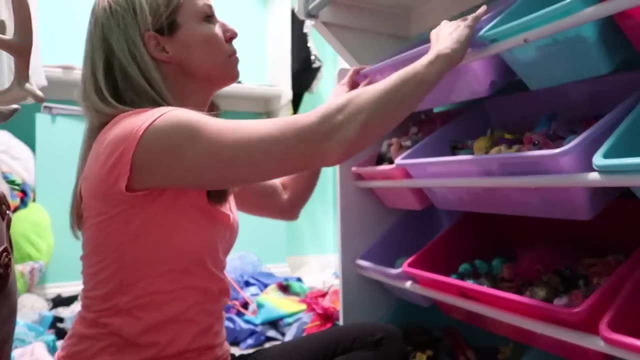 more to do, so much more to sort through, and I'm so tempted to just kind of pile everything in and walk away and be done with it. but I'm trying to motivate myself to keep with it and let's get this done and let's do it right. but let 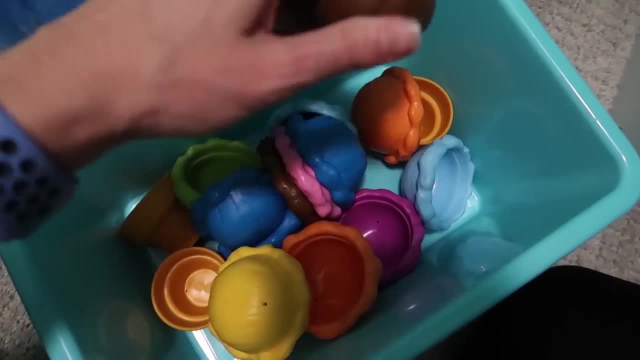 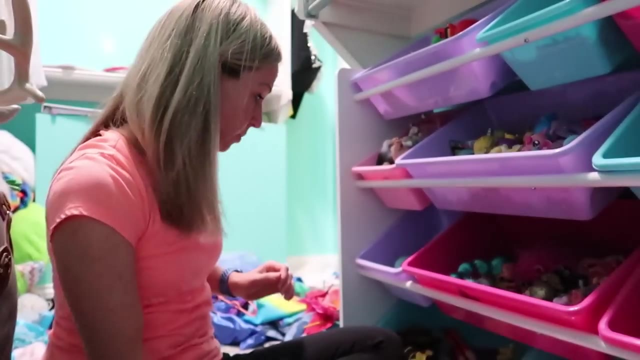 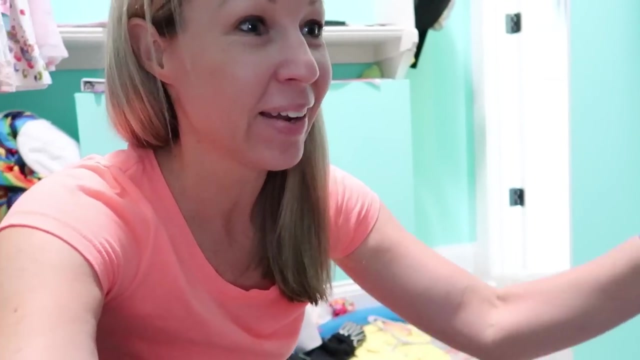 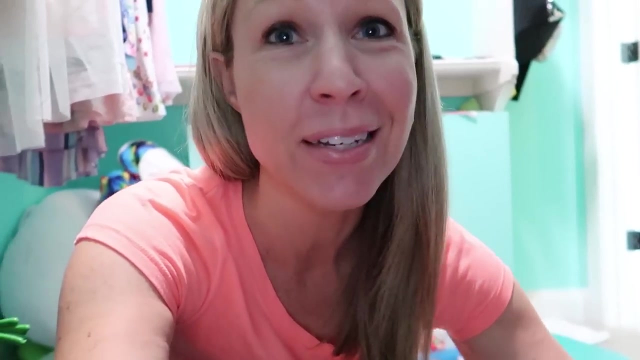 me tell you it is hard right now because I am wanting to be done. I have this big storage shelf over here in my closet that we actually use when we did our toy makers studio and I have all of our toys sorted by category so we have like our OMG pets in here. we have a big container of Wells, we have cloudies. 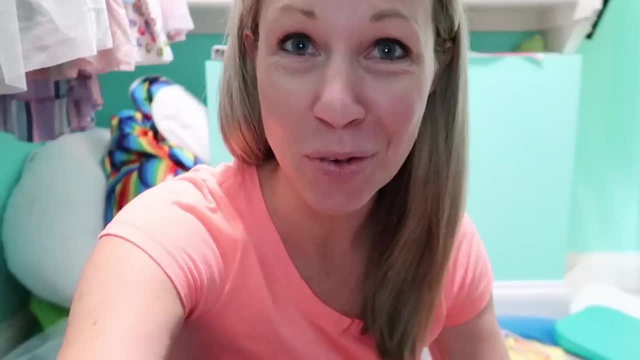 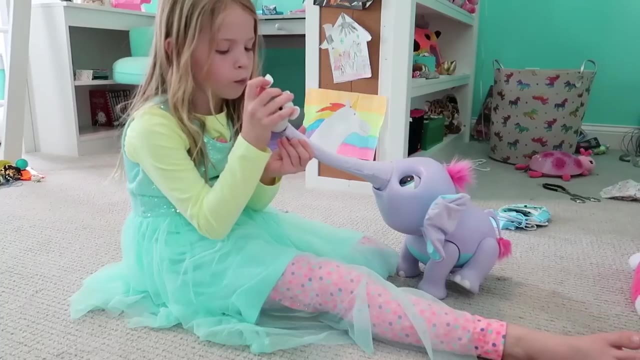 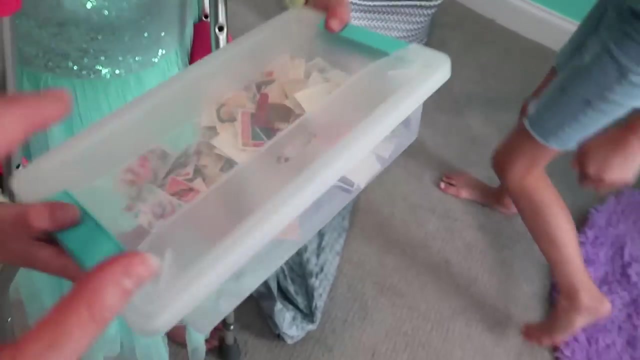 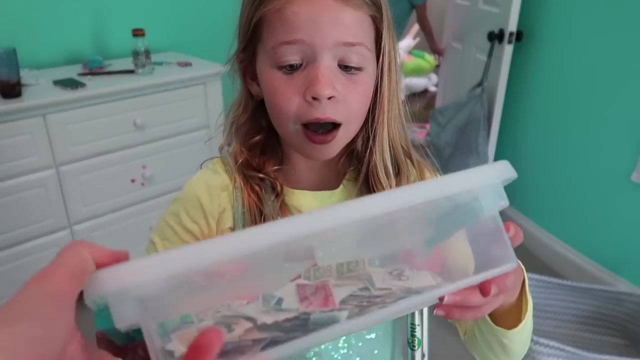 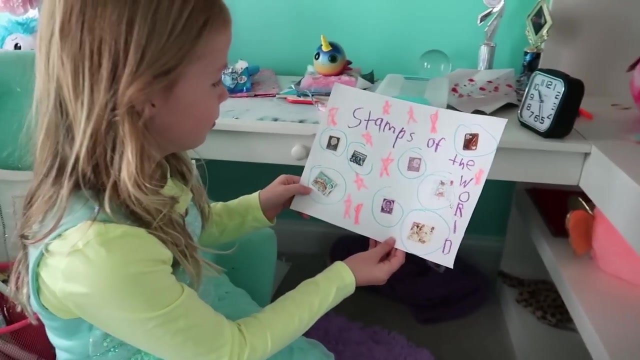 so I'm doing my best to keep them organized but still have them accessible for when friends come over and they want to dig into all these fun things. yeah, here's another thing. we used a bunch of stamps for an escape room video, but we don't need stamps, do we? you don't need all these stamps. oh so for art projects. 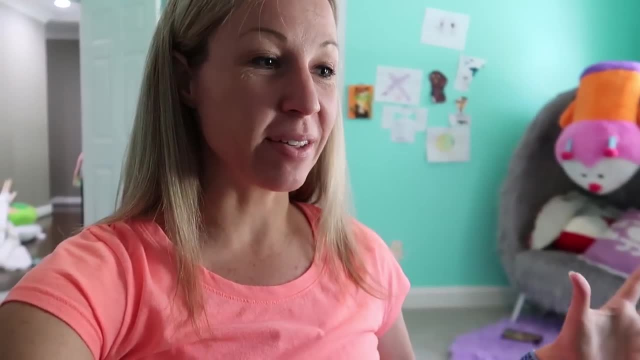 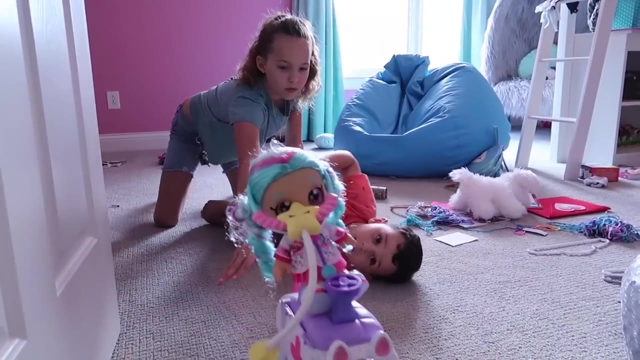 yeah, okay, well, maybe we can save the stamps in our art bin downstairs, and is that work? yay, all right, stamps go in the art bin and I repurpose them. apparently, Colin has decided to join the cleaning action, which I'm not sure what that is, so I'm just gonna go ahead and do it right now. so I'm just gonna go ahead and do it right now. so I'm gonna go ahead and do it right now, and I'm gonna go ahead and do it right now. so I'm just gonna go ahead and do it right now. of course is super helpful. 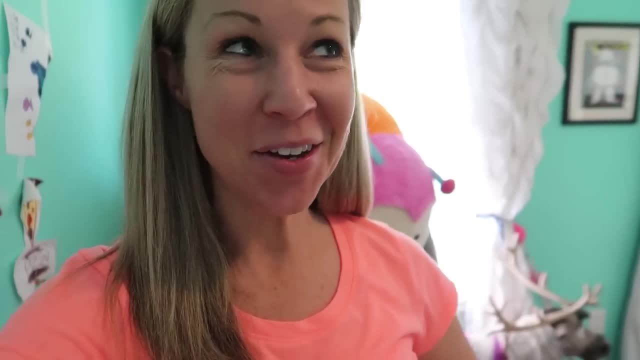 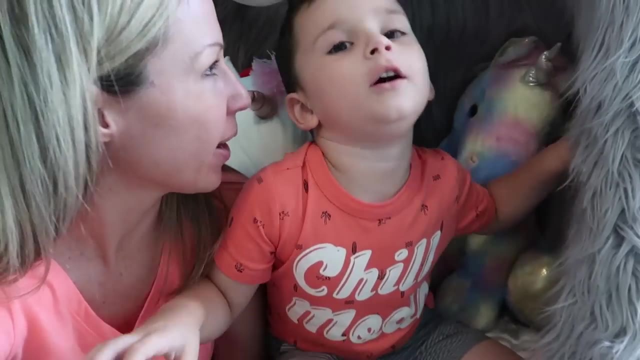 and that's just what we use. with another four-year-old walking around the room making more messes as we clean up the messes, Are we gonna clean your room next? Yeah, Yeah, Oh goodness, Colin's room actually isn't. 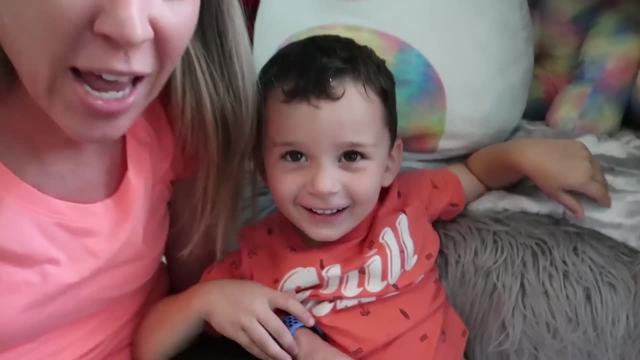 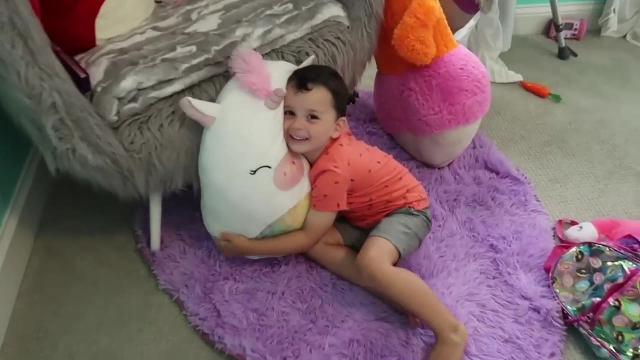 well, nearly as messy as the girls'. Your room's not this bad, is it, buddy? No, it's not, Colin. we just picked all this up, buddy. We gotta put it back now. Back up here, Come on, no. 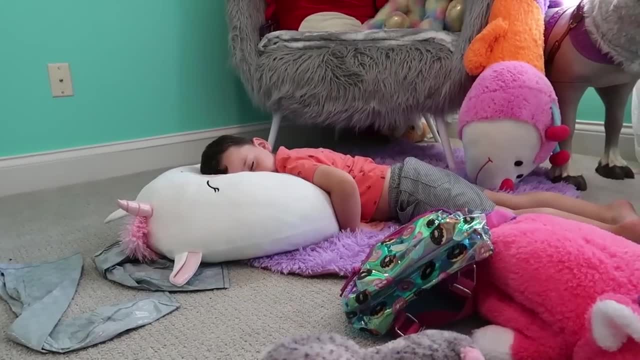 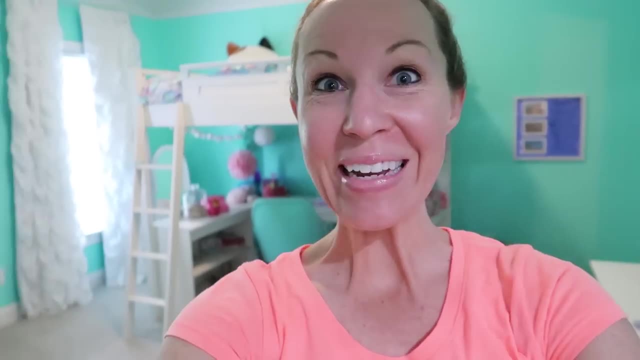 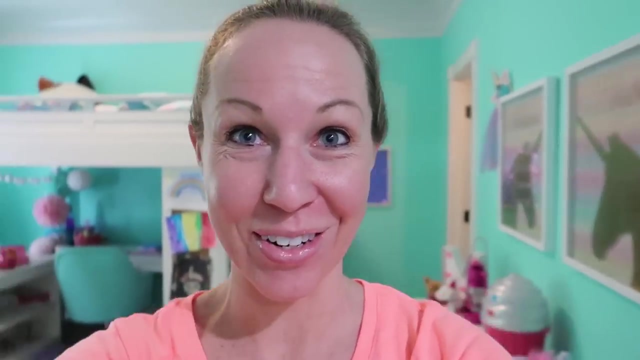 You're making a mess. Yeah, meh, We finally did it, guys. It has been five and a half hours since we started cleaning the bedrooms and it's done. I'm gonna show you a quick tour of Maya's room. 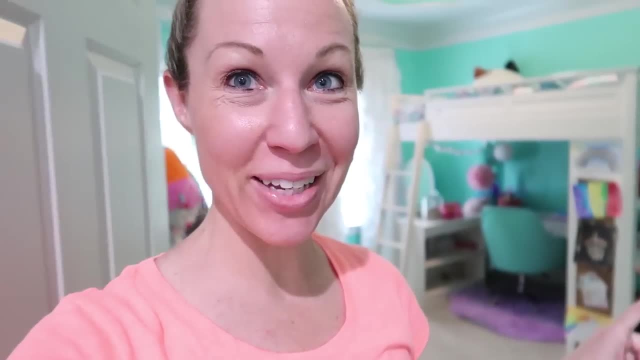 and then Addy's gonna show you a tour of her room. I haven't even seen the finished product yet, because she's been working so hard. Check out how clean Maya's room is right now. I don't think it's been this clean. 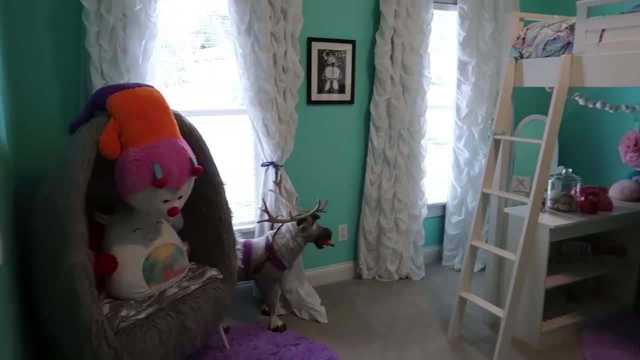 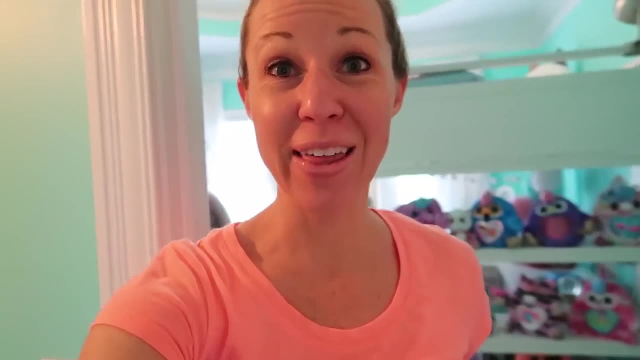 since we moved in, probably She's got all of her favorite things displayed here, and the part that I still can't believe is the closet Guys, it isn't perfect, but it's gonna be okay. I'm gonna show you the closet. 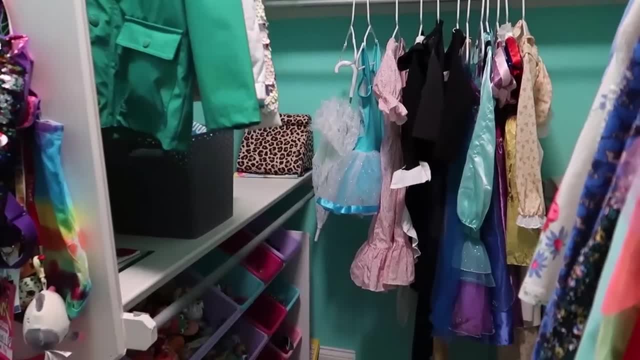 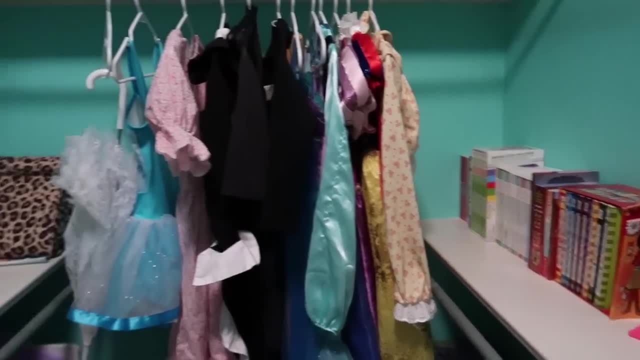 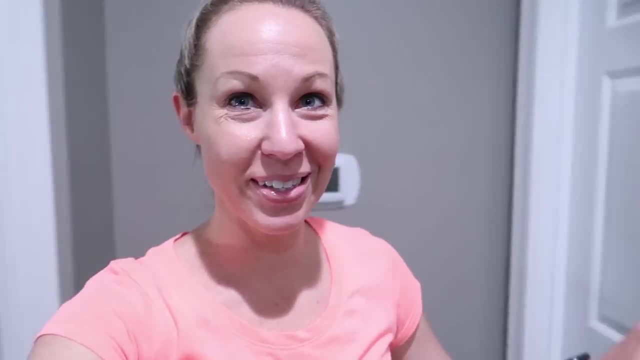 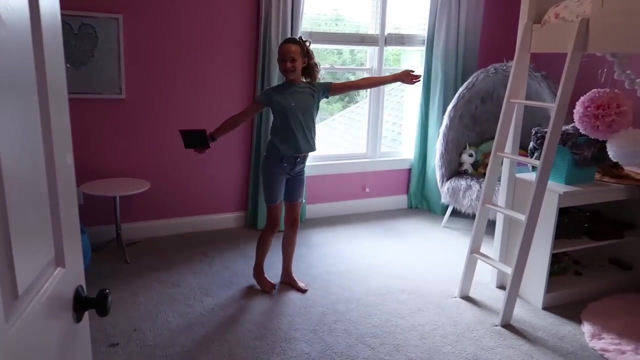 books, organized some toys up here. It looks amazing And I'm officially exhausted over that, but I am super excited to see Addy's room, so let's see: Welcome to my room. Wow, Addy, It looks so good. 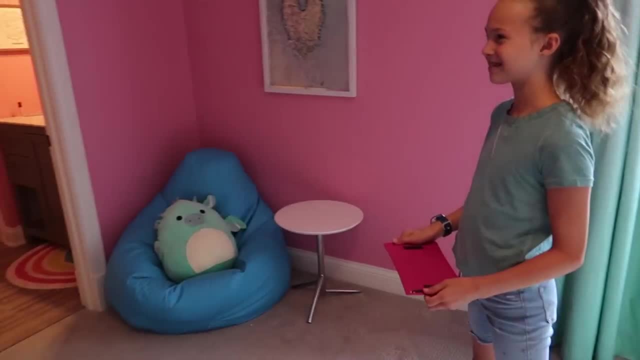 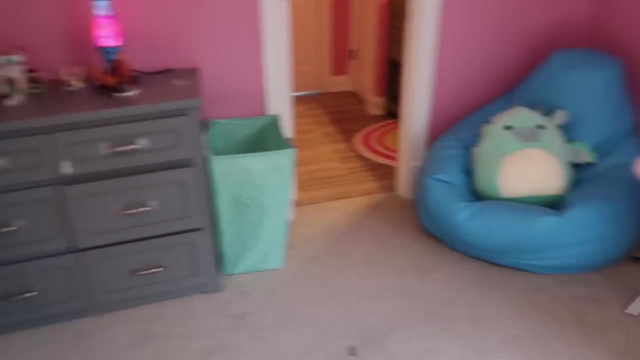 It looks so good, So so clean. We've got a lounge section over here now, and she moved her dresser over to this corner. Addy, this is looking pretty good. Yeah, What's your favorite thing you did in here? 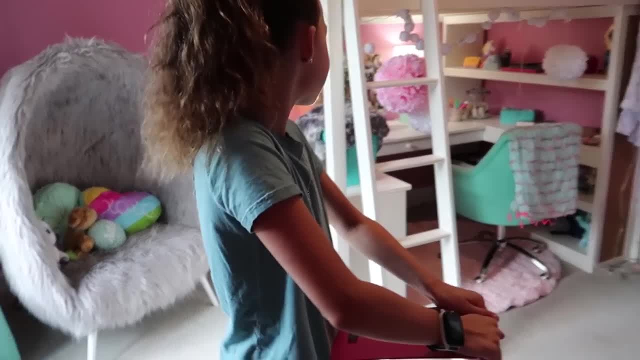 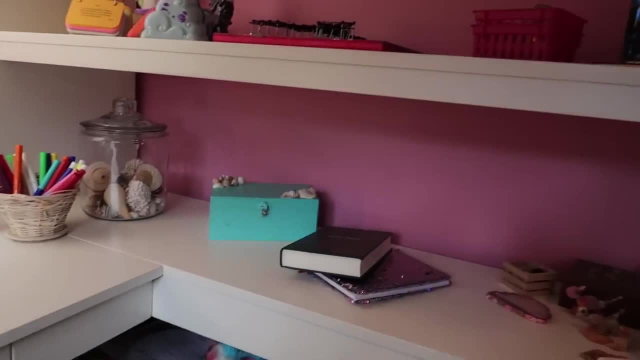 Or what took the most time: Organizing the desk. Organizing the desk, Yeah Well, it looks pretty good, Addy, I'm proud of you, girl. Addy's dresser used to be right here, but she's moved it. 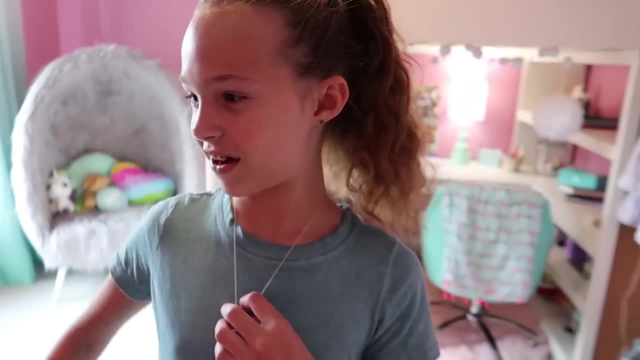 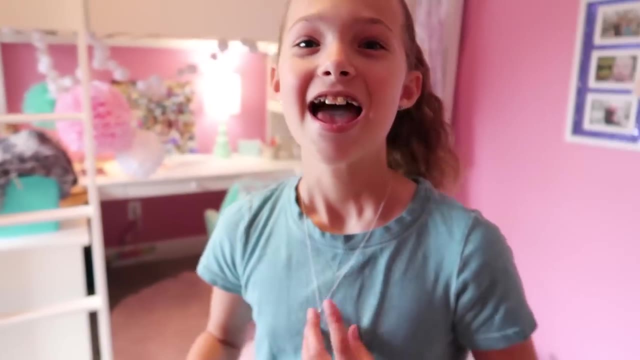 And Addy, tell us what you're gonna do in this spot. Well, later on I won't have the beanbag chair there and I'll put my gaming set there. That's right for your gaming channel. What's your new gaming channel, Carl? 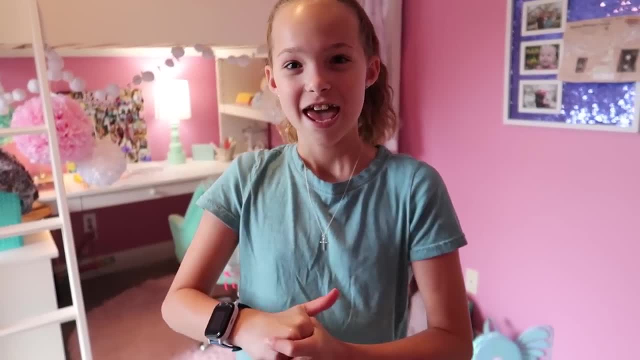 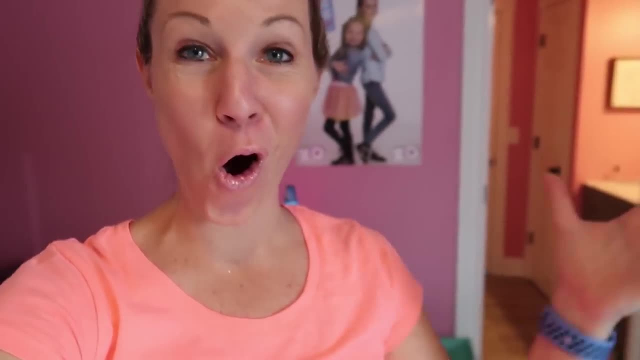 It's called XOXO Gaming, so you can just go scroll down to related channels and XOXO Gaming will be there. Please subscribe. Addy has been dying to have a gaming channel and it's really all her Like. she's doing it, she's planning it. 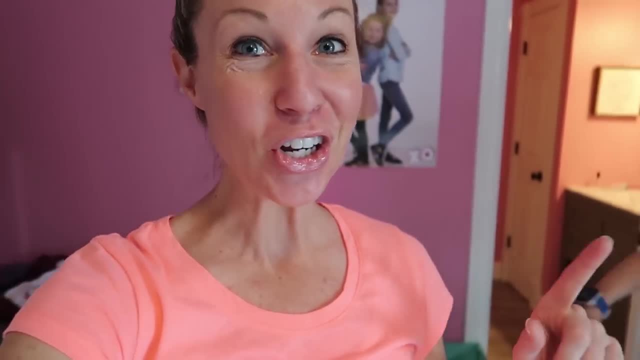 and I'm pretty impressed. She's doing a pretty good job. It just started, so make sure you, you know, make sure you subscribe to XOXO Gaming. And what type of gaming are you doing on it? Roblox Gaming. 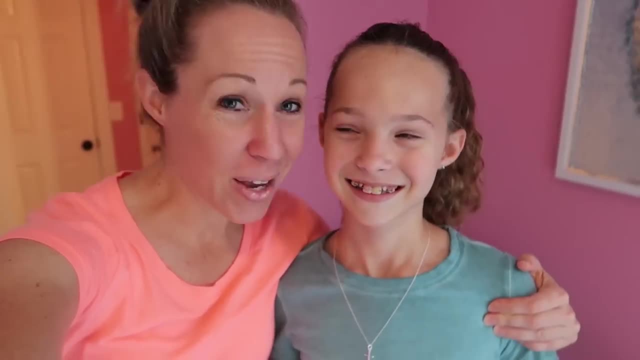 Your favorite? huh, Yes, my favorite. Well, good job, Addy. We got it done. Yes, It took a long time, but we did it. Yeah, Does it feel good to have a clean room? Uh-huh. 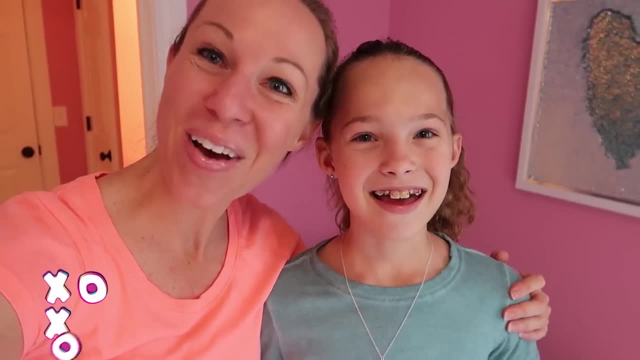 It always feels so good. I know. All right, what are we gonna tell our viewers? XOXO, Bye, Bye.